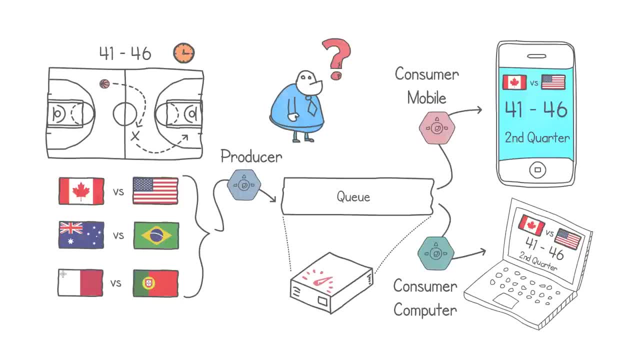 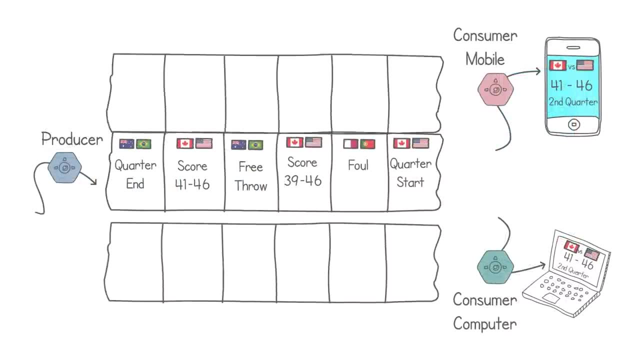 But how do we go about distributing a queue data structure? By its nature, the items in a queue follow a specific ordering. We could try to randomly distribute the contents of the queue onto multiple ones. If we do this, our consumers might consume the updates in the wrong order. 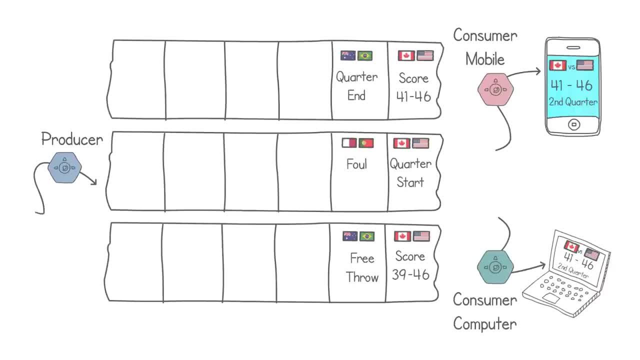 This would result in inconsistencies, For example, the wrong scoring being displayed across the channels. One solution is to let the application specify the way to distribute the items in the queue. In our example, we could distribute the items using the match name, meaning that the updates. 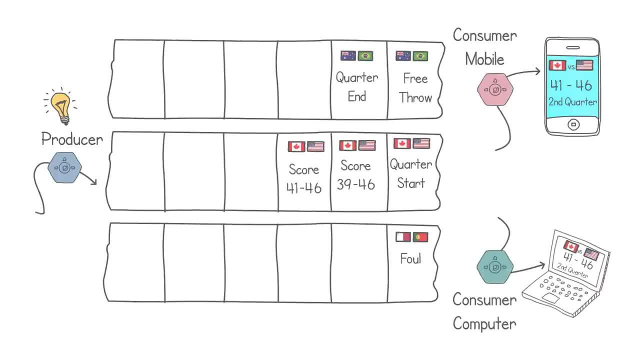 coming from the same match would be on the same queue. This strategy would maintain an ordering per basketball match. This is the basic, fundamental difference of Kafka from other messaging systems, That is, items sent and received through Kafka require a distribution strategy. Let's have a look at some more detail and terminology used. 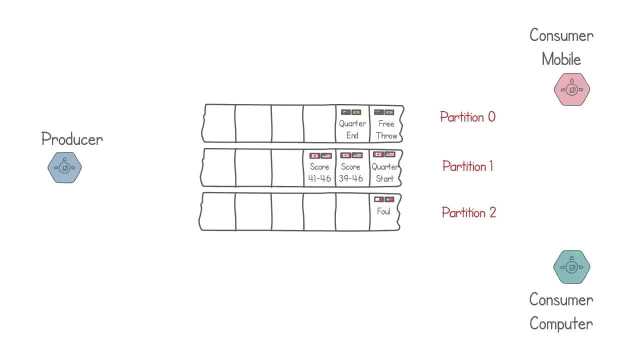 In Kafka, each one of these queues is called a partition and the total number of partitions is called a partition count. Each server holding one or more of these partitions is called a broker and each item in a partition is called a record- The field used to decide which partition the record should be stored. 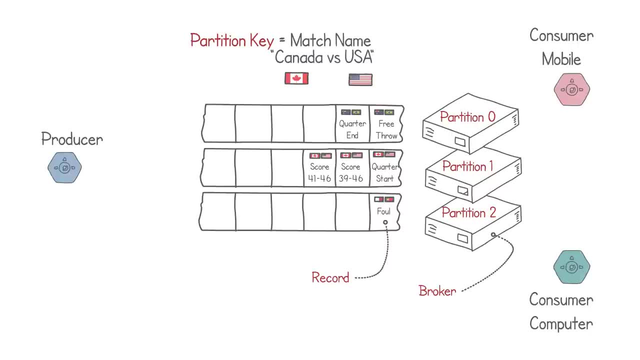 in is called the partition key. It's up to the application to decide which field to use as a partition key. If no key is specified, Kafka simply assigns a random partition. A grouping of partitions handling the same type of data is called a topic In order to identify. 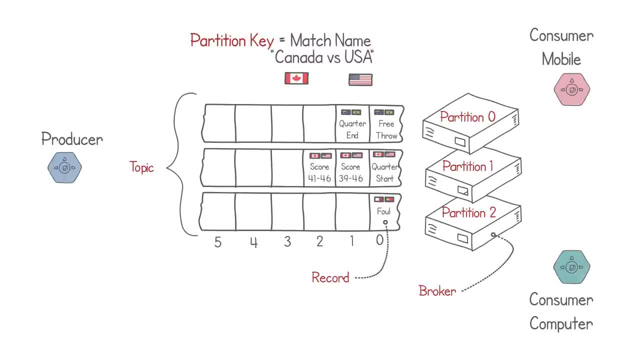 each record uniquely. Kafka provides a sequential number to each record. This is called an offset. Essentially, a record in a topic is identified by a partition number and an offset. In our application, since we have now distributed our data in the topic using the name as the partition key, we can now also parallelize our consumer applications. 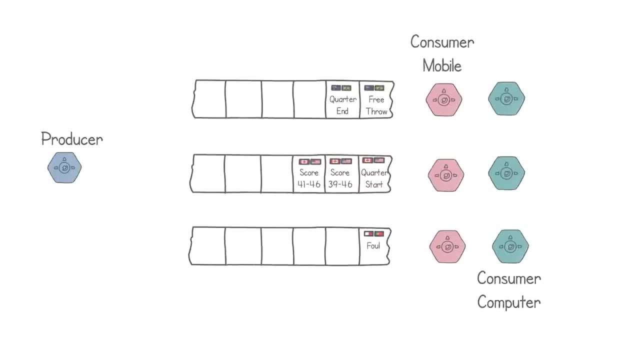 Having one consumer per partition guarantees ordering per game. Consumers can live on one machine or distributed amongst multiple ones. One important concept in Kafka is that consumers are very lightweight and we can create many of them without affecting performance. This is mainly because Kafka only needs to maintain the latest offsets read by each. 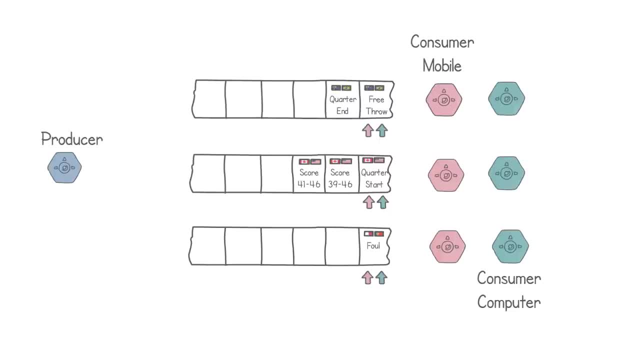 consumer. Typically, consumers read one record after the other and resume from where they left after a restart. However, in Kafka, it's up to the consumer implementation to decide on how to consume records. It's quite common to have consumers to read all the records from the beginning on startup, or to read the record in different orders, such as reading: 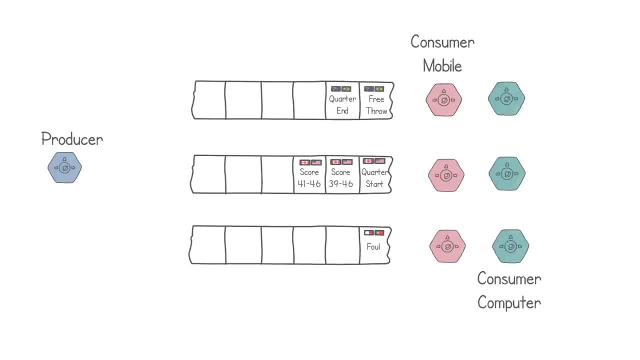 back to front. for example, In Kafka, each consumer belonging to the same consumer group do not share partitions. This means that each consumer would read different records from the other consumers. Multiple consumer groups are useful when you have different applications reading the same contents. In our example, we could have a consumer group called mobile and. 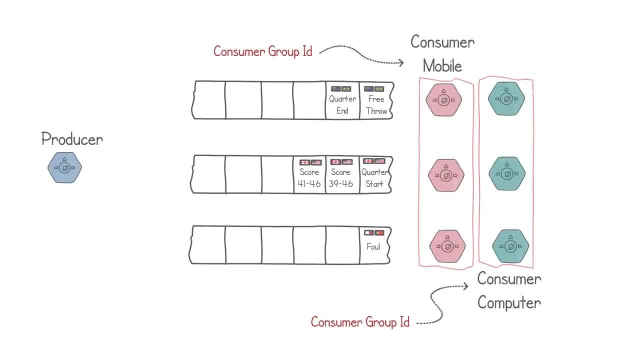 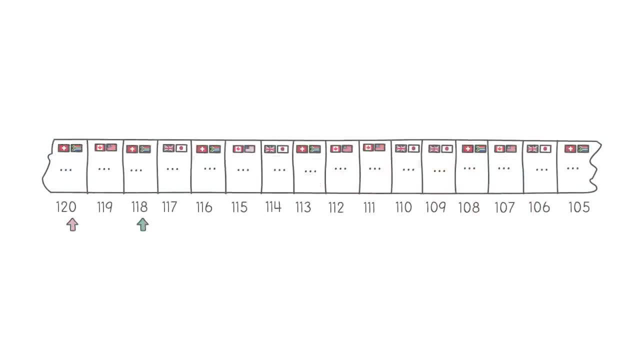 another consumer group called computer. These groups will read the same records but update different channels. Each consumer in these groups will have separate offset pointers to keep track of which latest record was read. If consumers can read using custom ordering, how can Kafka determine that a record has been consumed and it can safely delete that record so it can free up space? 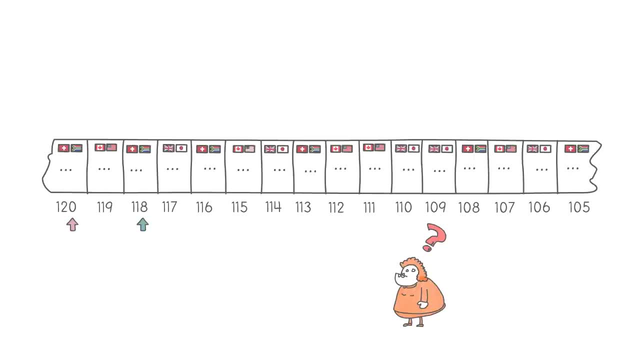 The answer is that Kafka provides various policies that allow it to do a record cleanup. For example, using a retention policy. you can provide a record age limit, say 24 hours, after which the records are automatically deleted, Using this policy if your consumer application is never down for more than. 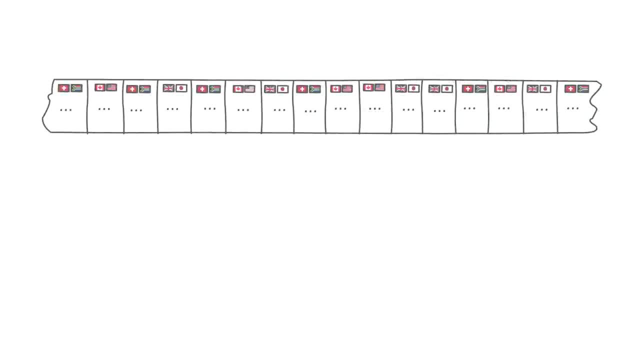 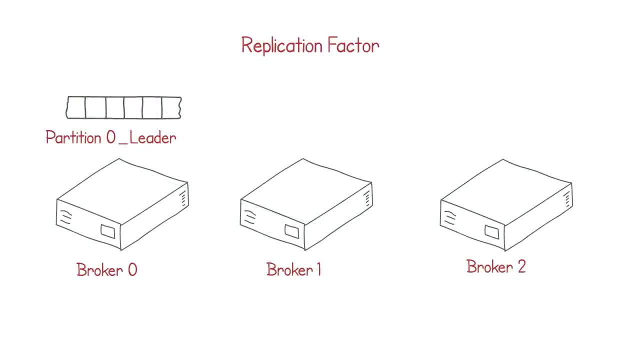 this age limit, no messages are lost. Another capability of Kafka is to store records in a fault tolerant and durable way. Each record is stored on persistent storage so that if a broker goes down, it can recover when it comes back up. Additionally, Kafka Replicates Partitions so that 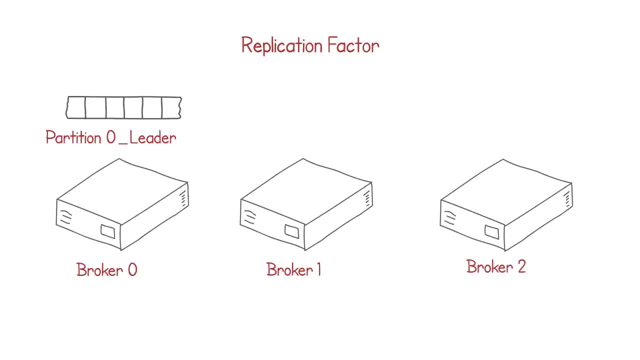 when a broker goes down, A backup partition takes over and processing can resume. This replication is configured using a replication factor. For example, a replication factor of 3 leads to 3 copies of a partition: 1 leader and 2 backups. This means that we can tolerate up to 2 brokers going down at the same time.